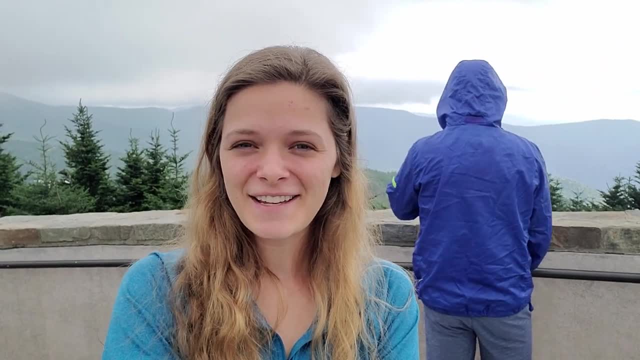 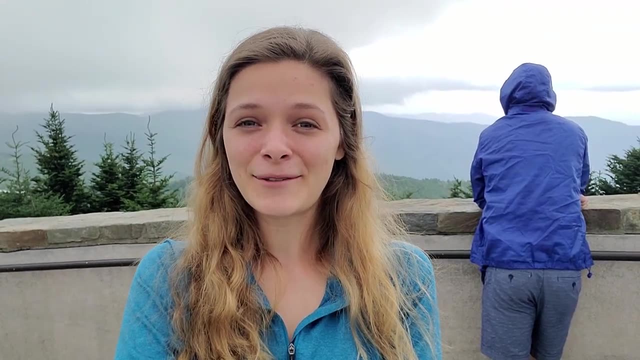 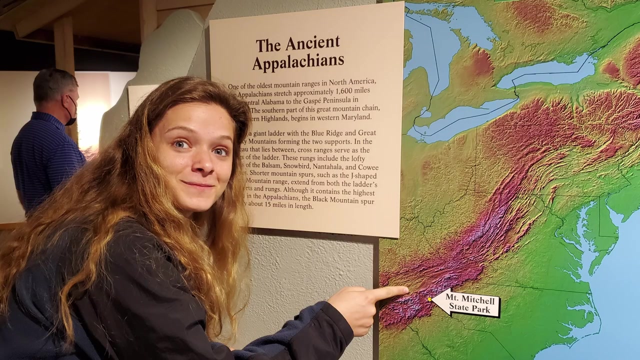 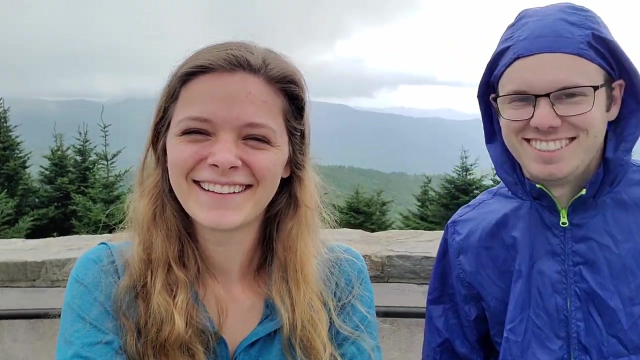 Hey and welcome back to another episode of What To Do. Today. we are at the highest point east of the Mississippi River. It's called Mount Mitchell. This place is absolutely stunning. There are actually a lot of things to do here and some really cool information and facts, So stick around to get the entire scoop Ridiculous. 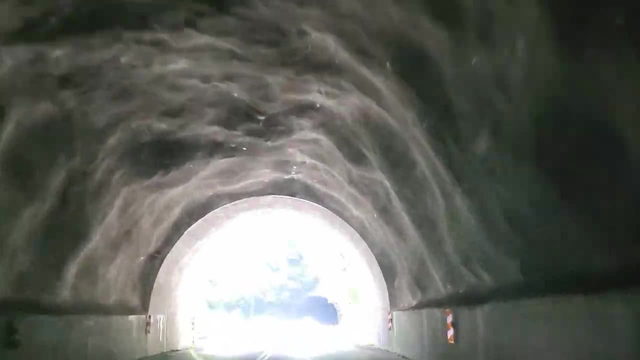 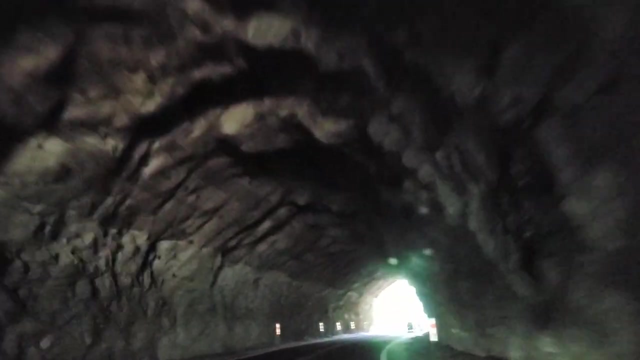 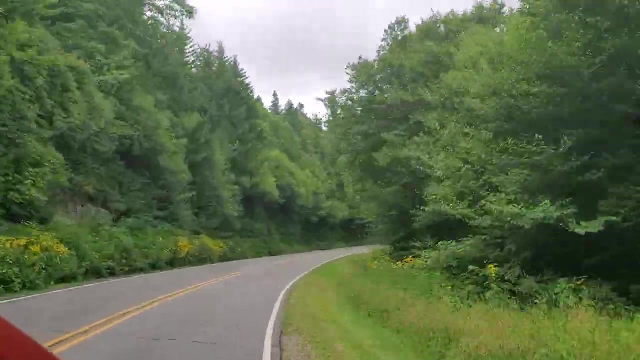 It's a double tunnel. Look at this. This is: oh, this is cool. This is super cool. It looks even better in the camera. Oh, that's awesome. On our drive up to the mountain they had an old time radio station narrating some interesting facts about Mount Mitchell. 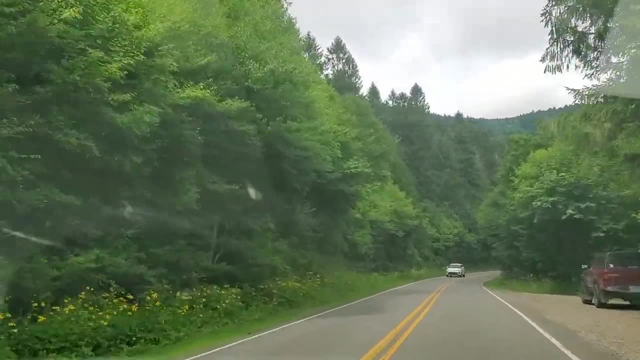 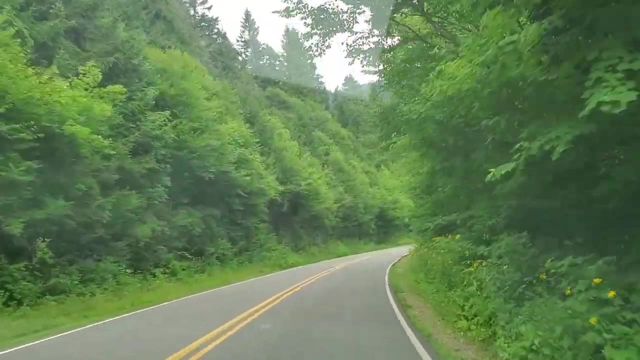 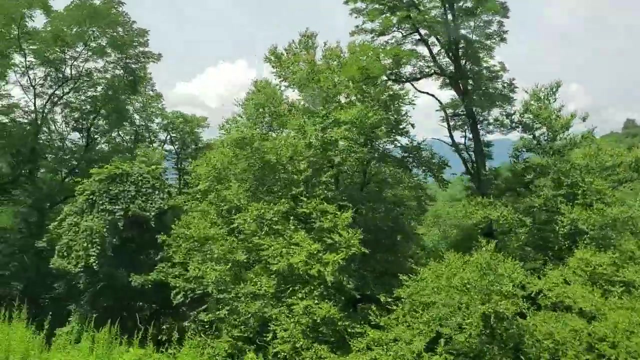 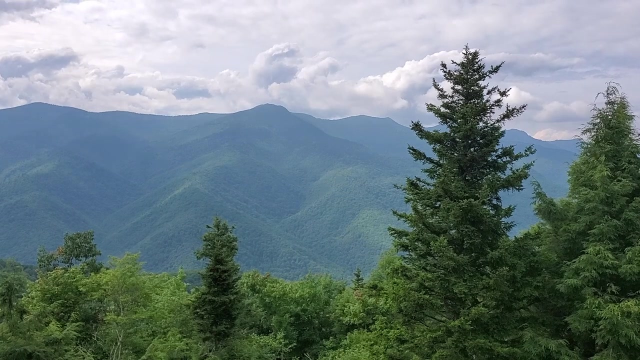 We hope you enjoy this old fashioned AM radio station, Just like Granddad used to At Blue Ridge Park. On Parkway mile marker 355,, you begin your ascent to what's been called the A-Cast of Appalachia At 6,684 feet above sea level. Mount Mitchell is the highest point east of the Mississippi River. 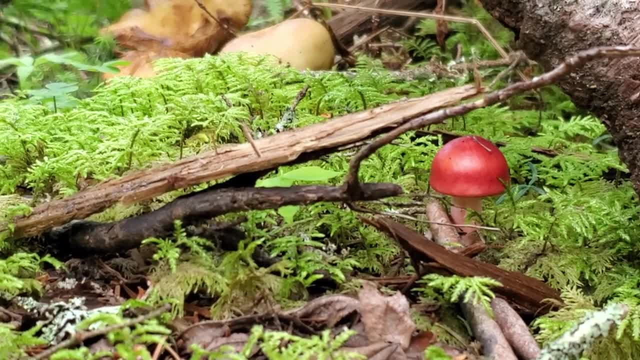 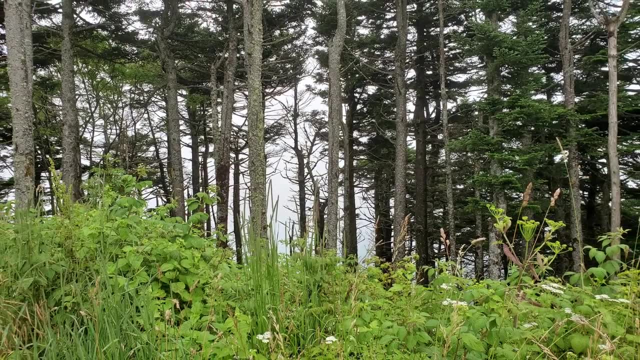 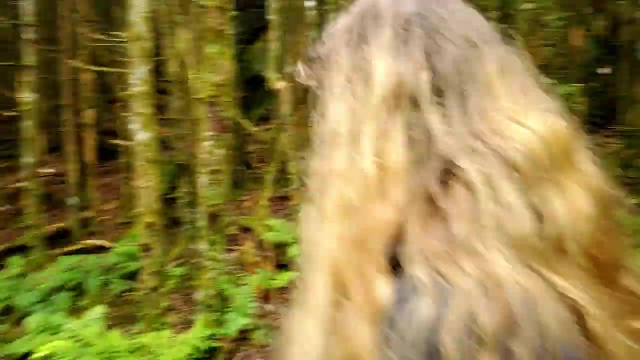 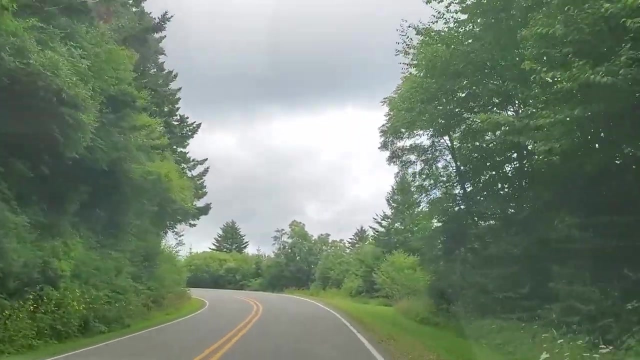 Driving up, you experience one of North America's most habitat, diverse stretches of road, with temperatures often 20 degrees colder than nearby Valley Town. The cool climate preserves a rare alpine forest that more resembles Canada than North Carolina. You'll find the park office and ranger station two miles up the road on your right, with maps, park information, restrooms and drinkable water. 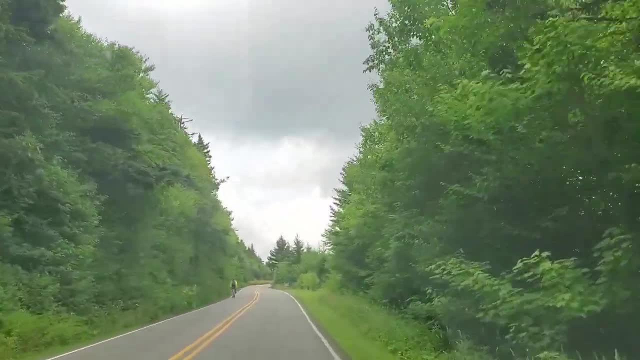 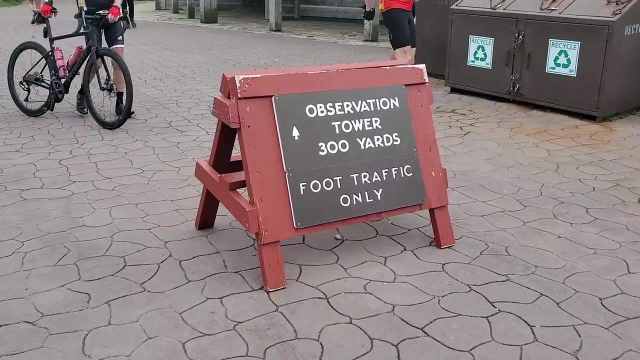 I'm glad they have restrooms. That guy's going to go fast down that hill. Come back in 2022 for some of the best apple pie on earth. Okay, We're going to go right this way. Did you bike all the way up? 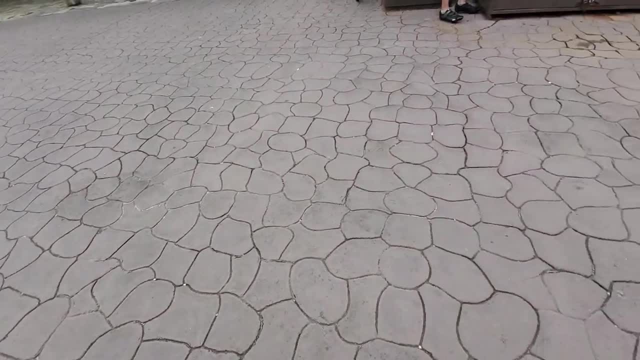 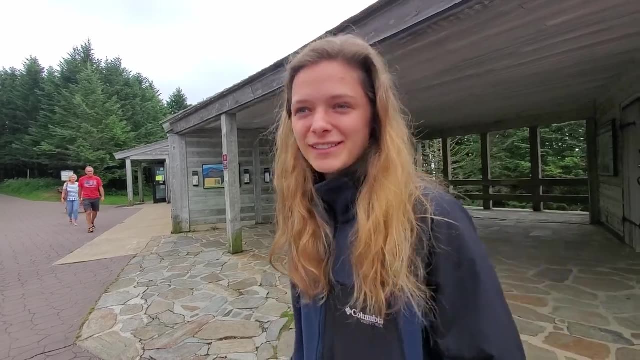 They carried his bike. He's lying on it Three-handed yards up. Do you think we can make it? If those bikers can bike 11 miles up this mountain? we can do this. So how did Mount Mitchell get its name? 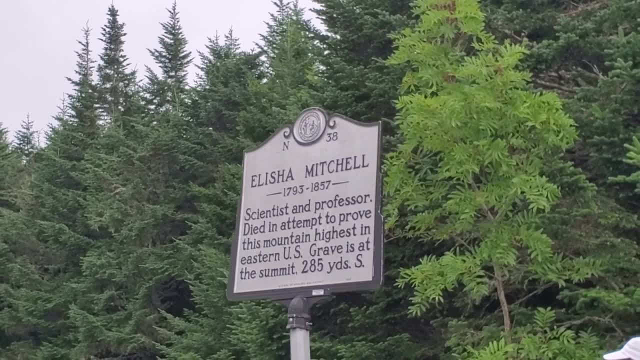 Well, the museum at the top will explain to us who Mr Mitchell was and why this mountain bared his name. We're also going to learn a few other fun facts. We're also going to learn a few other fun facts. We're also going to learn a few other fun facts. 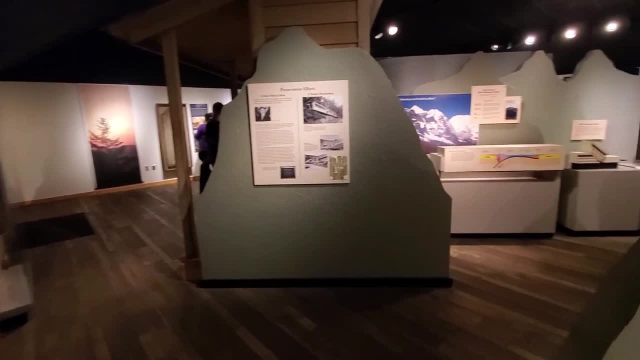 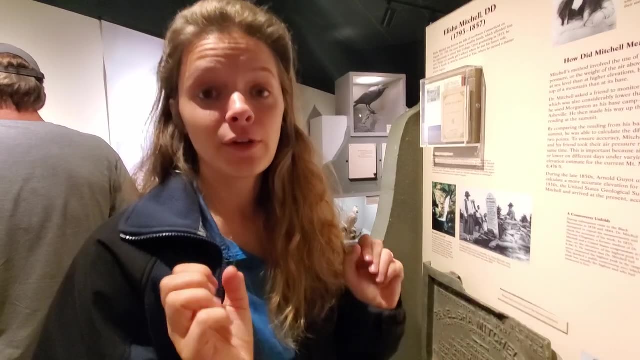 This is cool. It's like really well established. This is cool. It's like really well established. There's like geology over there. There's like geology over there. There's like geology over there. Okay, so Mitchell was somebody who studied this mountain. 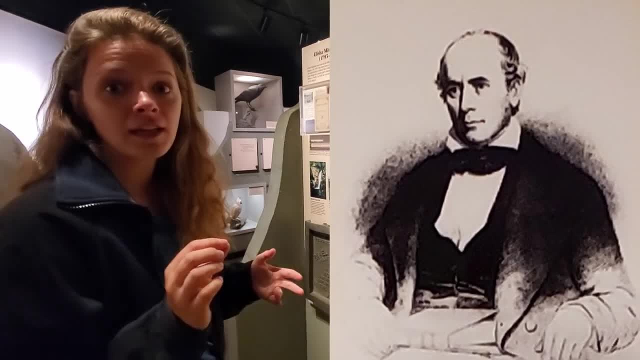 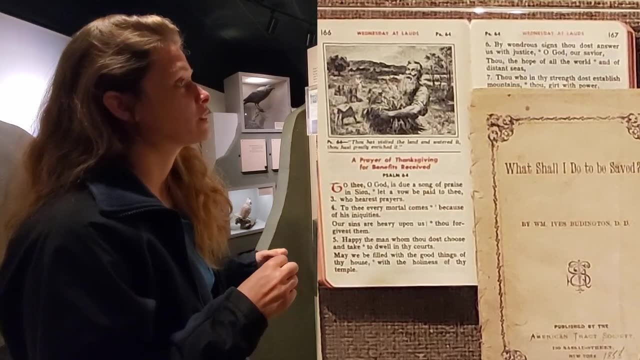 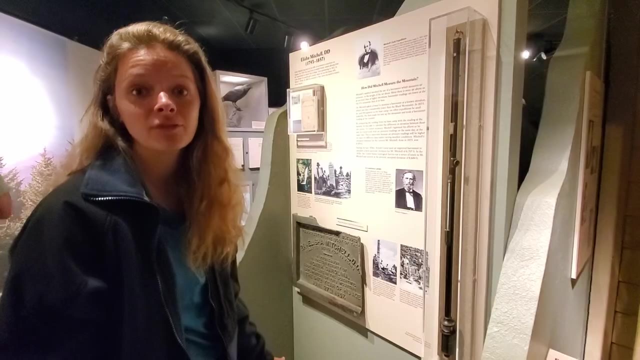 Okay, so Mitchell was somebody who studied this mountain, And he was a mathematician and a programmer, I guess- And he came to Mount Mitchell and started measuring it with this barometer And he said that Mount Mitchell was the tallest mountain. And this surprised everyone, because everyone thought that it was Grandfather Mountain which was the tallest mountain. 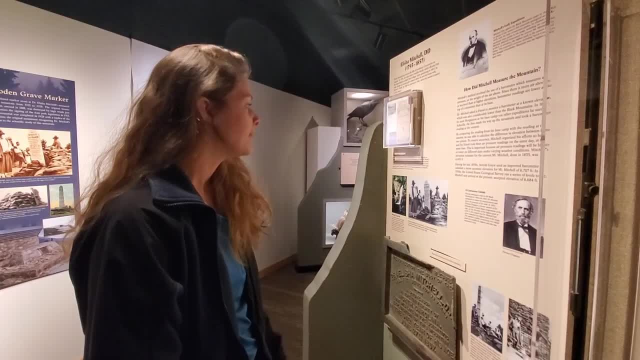 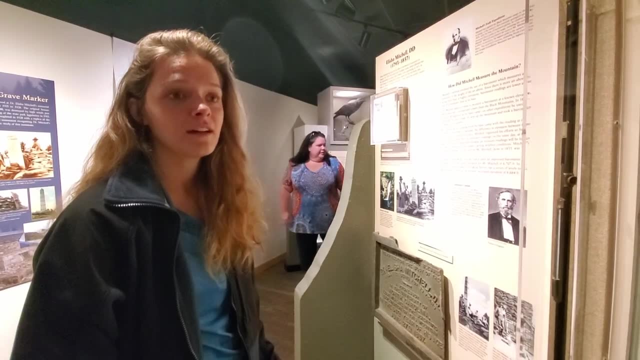 It was a controversy. It was a controversy over the elevation, And then he kept on coming back to gather more data And then, sadly, one day he came back and he fell off a waterfall, knocked his head, went unconscious and then drowned in the waterfall. 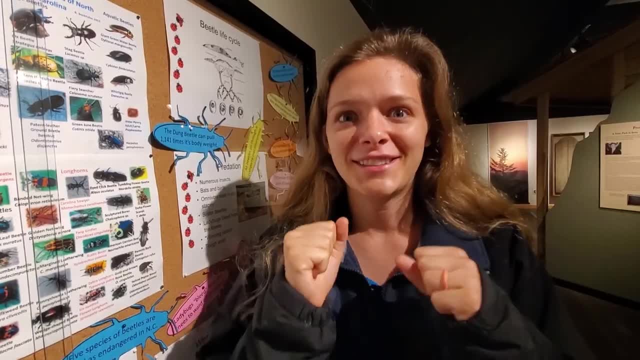 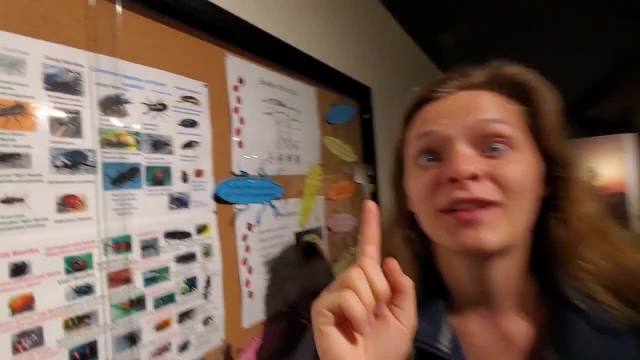 And that's how he died. Okay, so there's this beetle called the Eastern Hercules Beetle And it's huge And it's here, And we didn't see it here, We saw it at home. So I'm going to show you that clip right now. 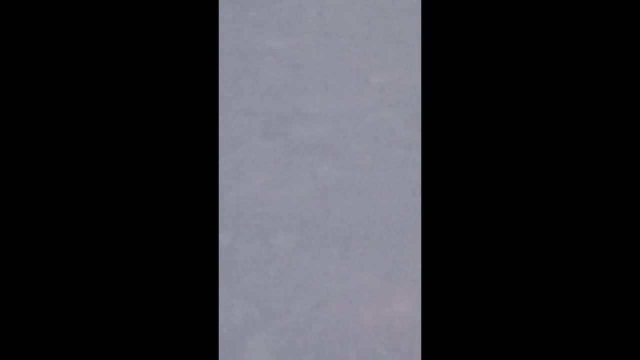 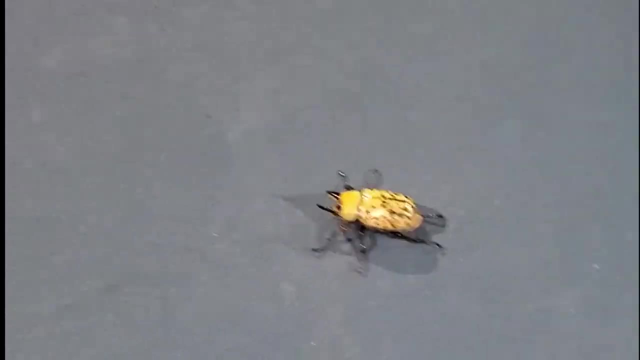 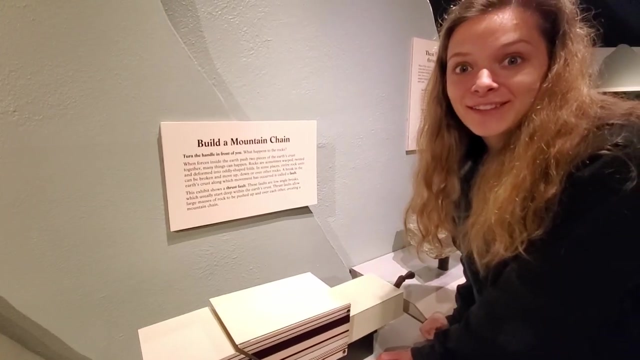 Oh, Oh, there it takes off. It's coming for you. I bet that big thing has lungs. You scared me, Okay. so this is how a mountain is made. You have these cracks in the earth called faults, And sometimes they'll be thrust up. 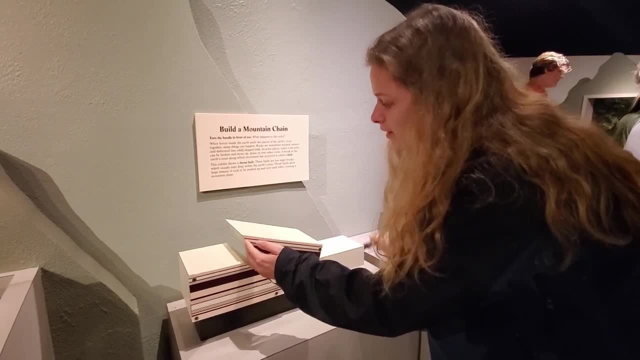 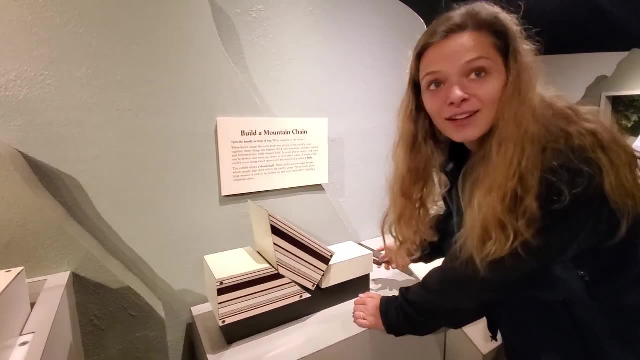 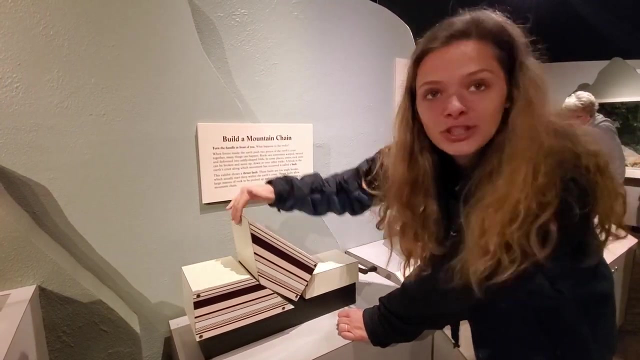 And they're thrust up. There's like this wall, And they're thrust up and make like these rigid things that are mountains. Isn't that cool? And so they say the Rocky Mountains are a lot younger than the Appalachian Mountains And you can kind of tell because the Rocky Mountains are sharper. 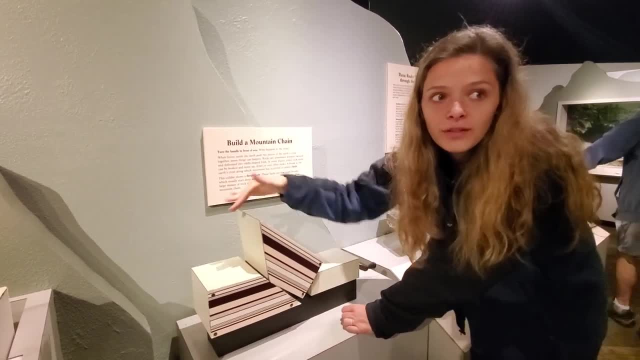 And the Appalachian Mountains are a little bit like smoother on the top, Like they've had time for the weather to wear it away. Oh, here we go. Welcome to Mount Mitchell's Summit Trail. Follow this moderate, paved 280-yard observation trail. 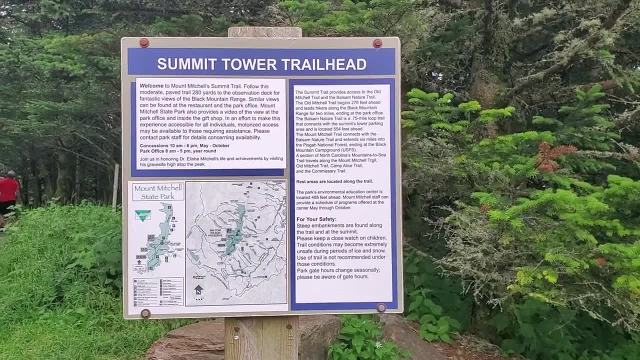 Fantastic views of the Black Mountain Range. Okay, to kind of give you an experience of what it's like up here Right now: I've been here before when it was really windy, But right now it's like really like oddly quiet. 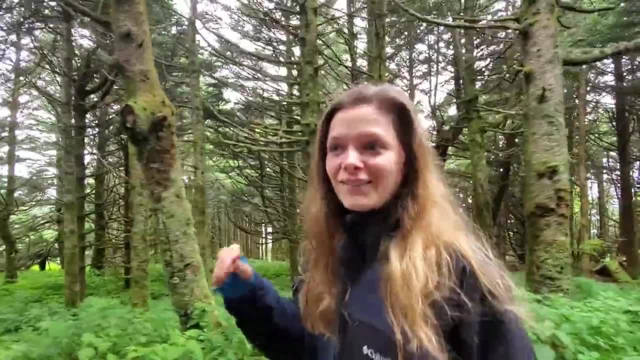 Like there's no wind And whenever people talk, it's not bouncing off of anything, It's like dissipates into the air. Can you see the fog? Yeah, That's so cool. It's really pretty, Really pretty Yeah. 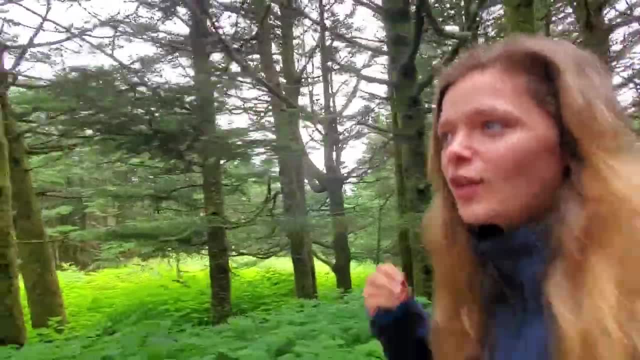 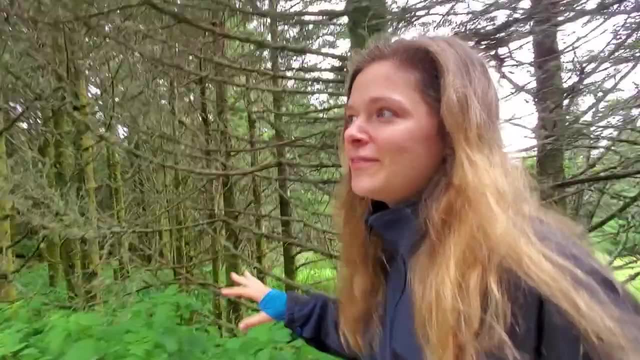 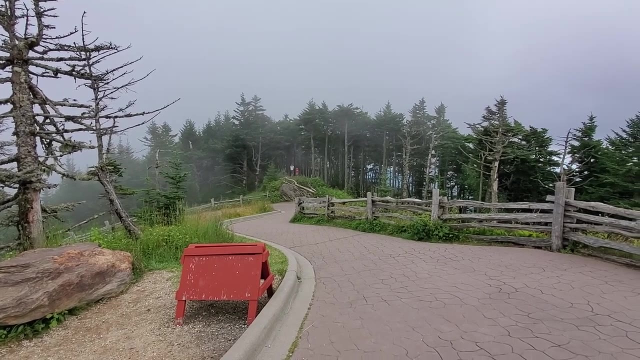 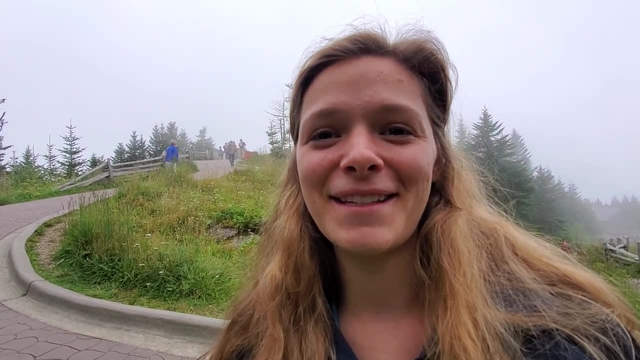 We're getting to the top of Mount MIT And the Haiyung Sun facing the west. It's like this blue star And then the smell is like fresh mountain smell. It's really cool. Another really cool thing about this place is there's tons of wildlife. 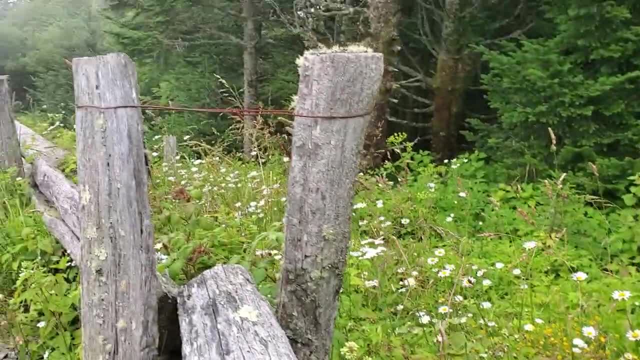 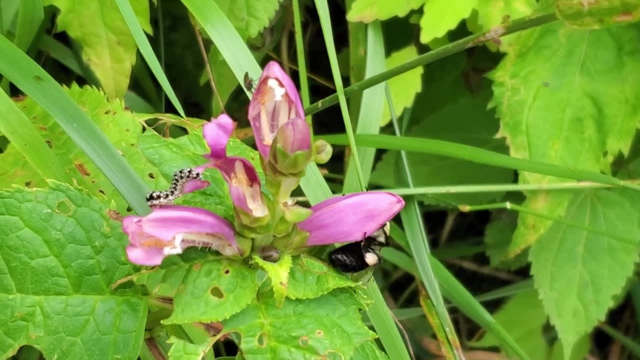 You guys go ahead. Volcano, Yeah Right, Yeah, Yeah, There's millions of� Yes, Yeah, Okay. Yeah, There's many kinds. Looks like they're proof and margin and so forth. Yeah, Not really, Maybe the mountain. 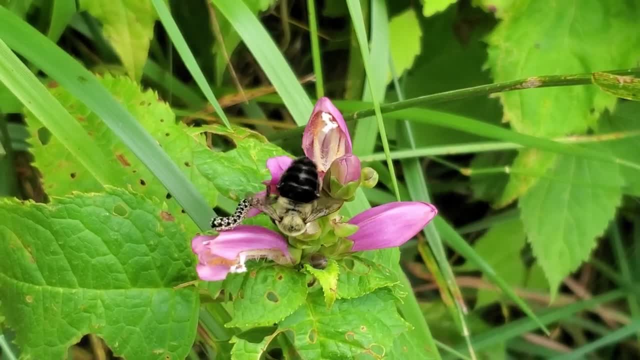 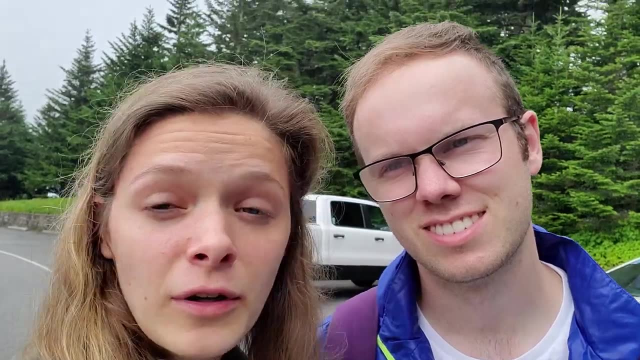 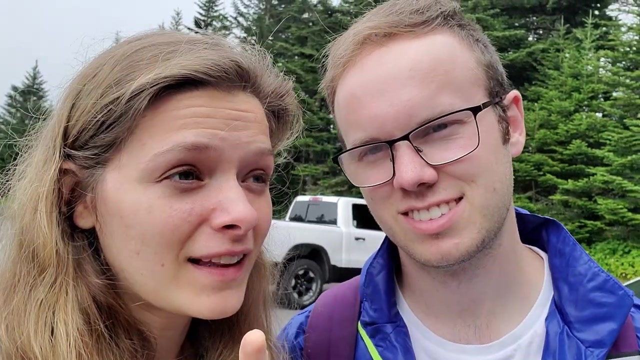 Oh, it's a bee. Oh, you pushed the cat out. We are interrupting this video with a very important announcement: that if you click that like button then you'll get to see more of this video, But only if you click that like button and you'll get to see the very end of the video. 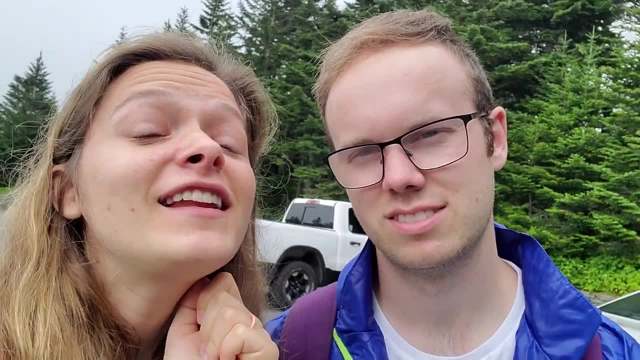 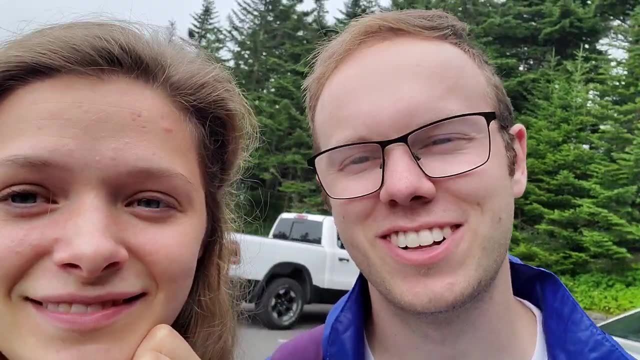 if you click that subscribe button, So do both, and it would help us out a ton and Well whether or not you still gotta get to see the video, but it'd be helpful. Oh, thank you for clicking it. 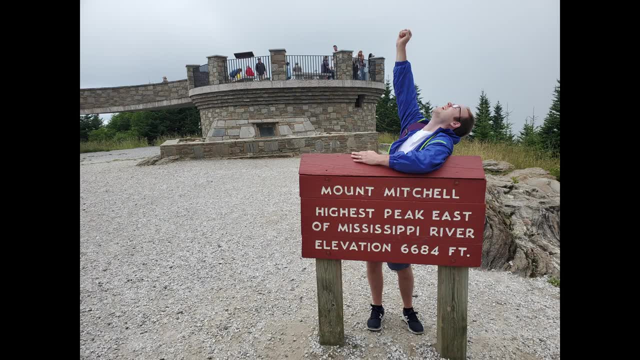 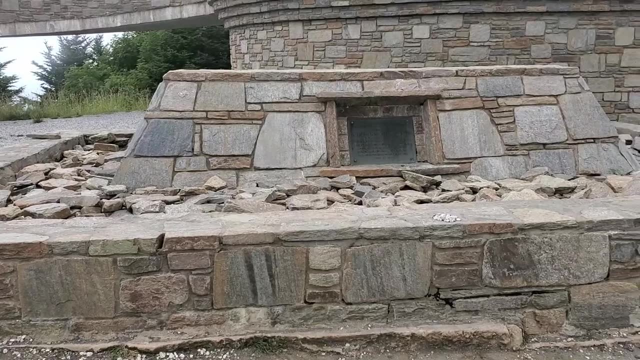 Now you will continue. When we finally made it to the top of Mount Mitchell, we didn't expect this, but behind us was Mitchell's Memorial. The owner of the mountain, Jesse Stepp, was a friend of his. Saddened by the death, Stepp built a memorial for Mitchell at the very top. 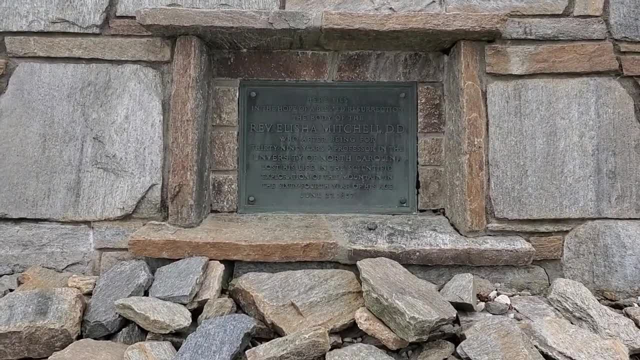 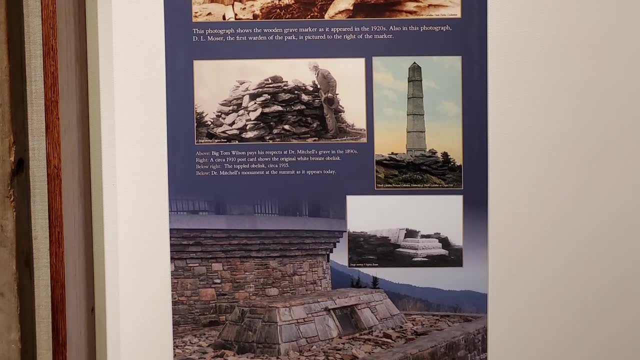 Eventually, Stepp sold all but this area to preserve Mitchell's memorial. Originally it was a wooden plaque, but the intense weather conditions blew it away, so they replaced it with something else, Something a little more durable. Elevation getting to you Will. 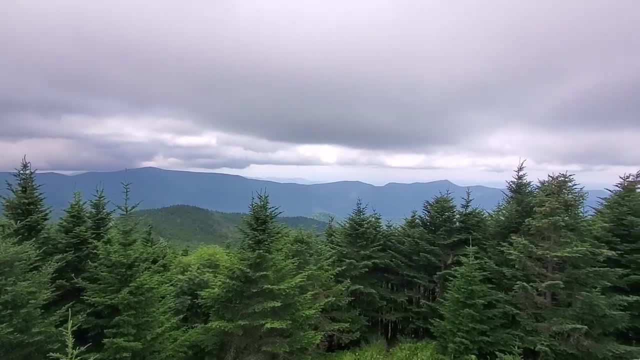 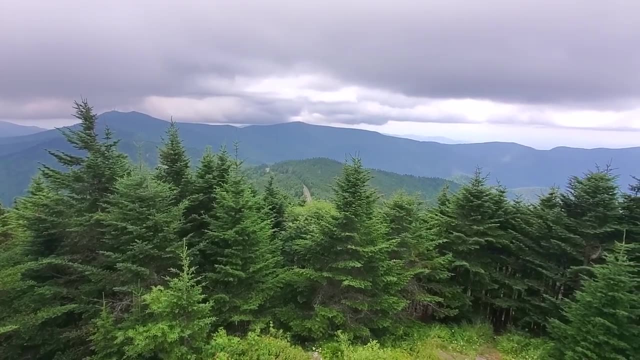 Wow, Those look taller. No, we're taller. We've been That road down there. that's the road we drove, No, I think so. You know, what's funny is we've been driving and like the whole time we're looking up at mountains.